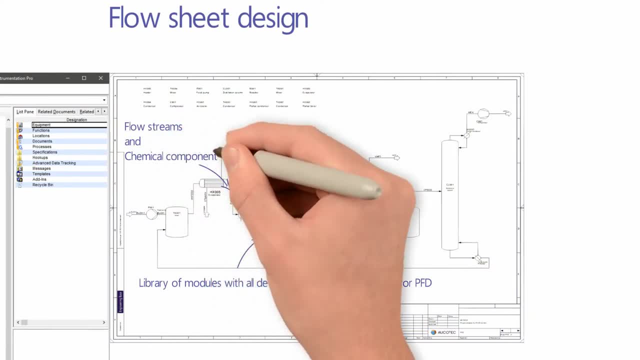 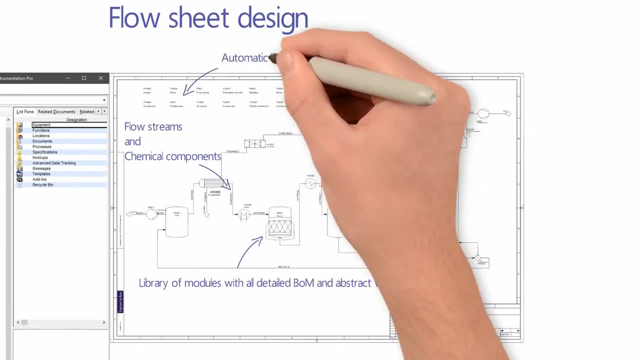 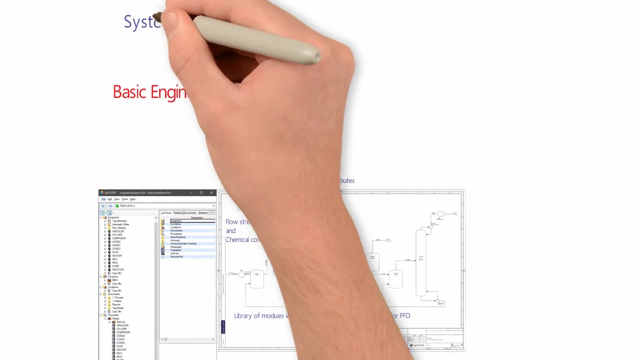 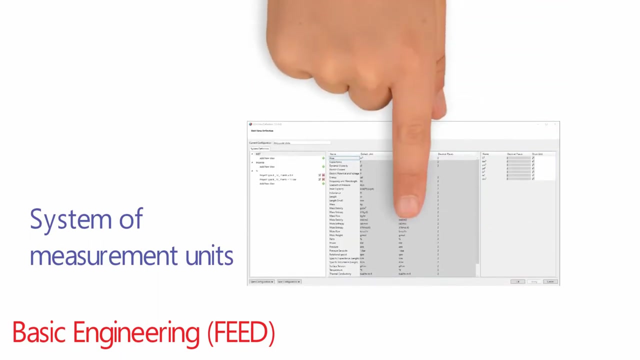 Attributes of flow streams and chemical components can be shown on streams. Attributes of unit operations can be listed automatically on the PFD. For the design of a process, various measurement units can be used. The system of measurement units, default values and available lists for users can be configured. 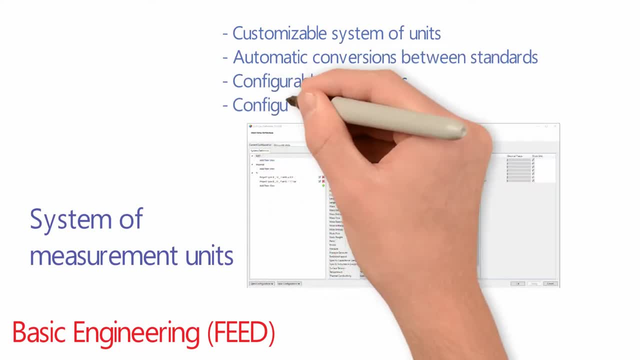 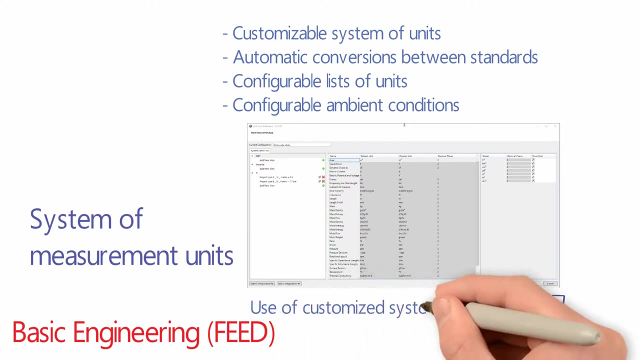 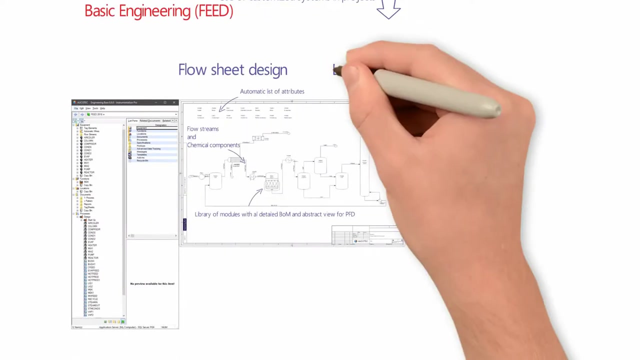 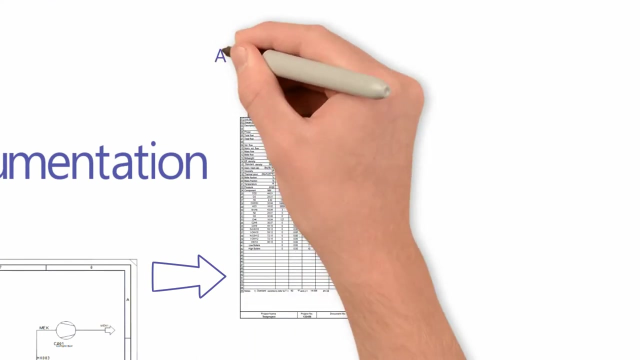 Units will be converted automatically and the ambient conditions of the project can be modified in the project settings. For each project, different custom measurement systems can be used. At any point in time during the design. documentation can be generated automatically. In the future, it's easier to see how many units can be used. 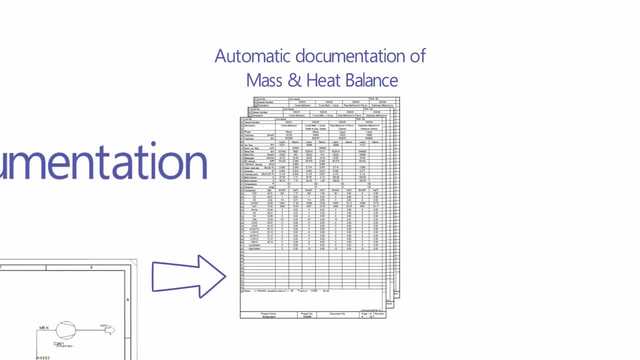 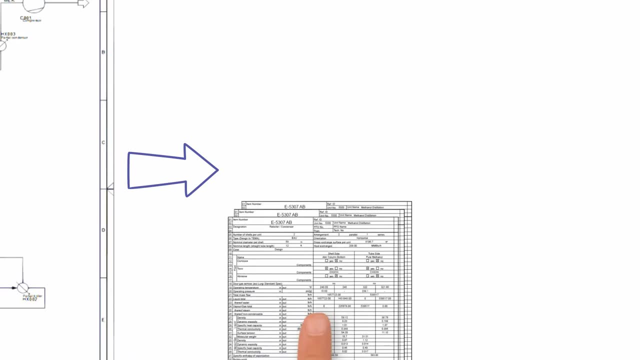 This documentation includes mass and heat balance sheets, equipment data sheets and a list of all the components required for a process. If the process is not very successful, we can easily give up a project because it is not in the best condition. Equipment data sheets. 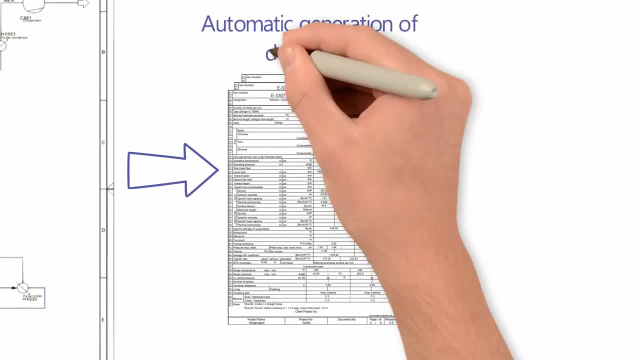 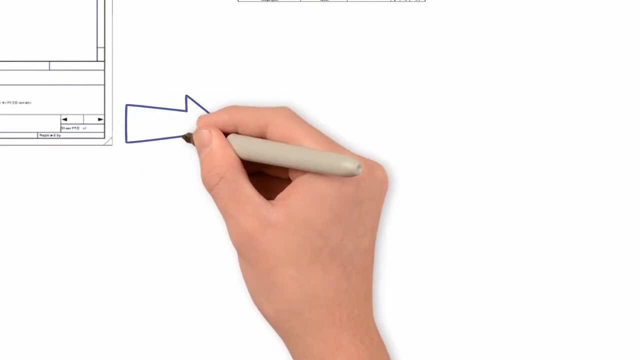 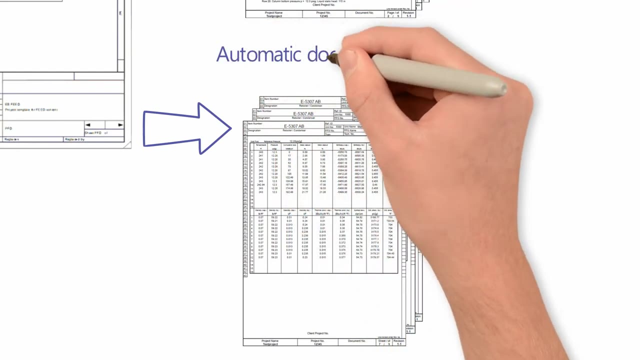 equipment data sheets and group data sheets can be used to process work. Uses of equipment data sheets are also available. Frequency measurement temperature, air temperature, temperature and humidity are included. …and curves and profiles data sheets. These documents will be consistent and will all change automatically. 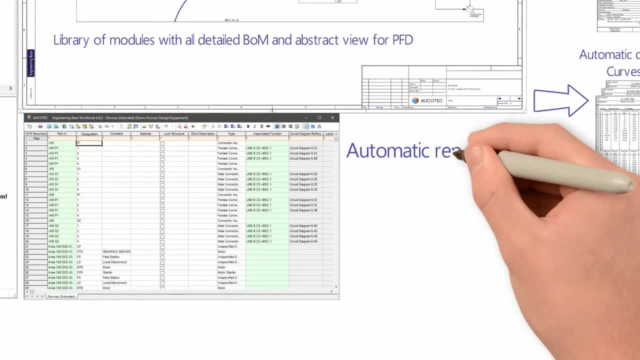 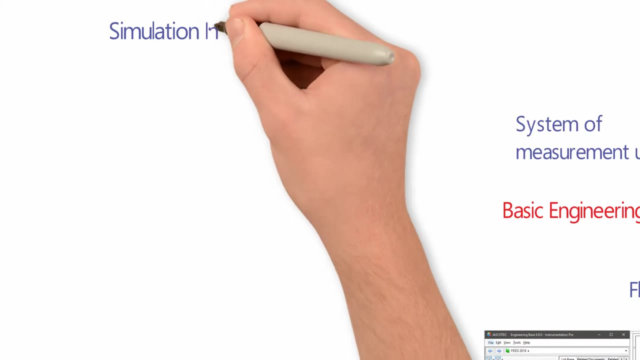 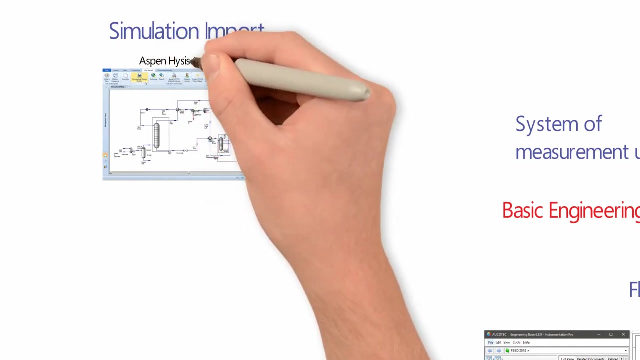 Various lists of data can also be generated and can be used for modifications. Process simulation: One of the most important sources of data in basic engineering is the process simulation tool From the Aspen HiSys simulation. a standard XML can be exported to the ECB.